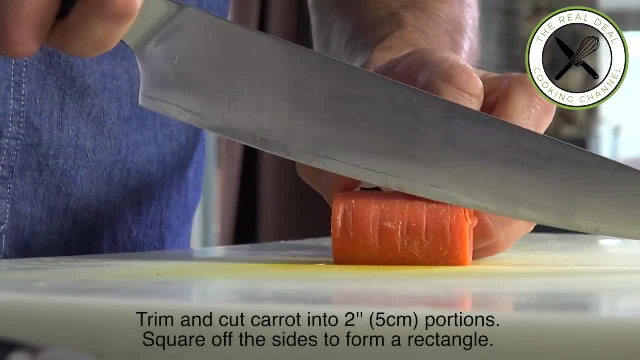 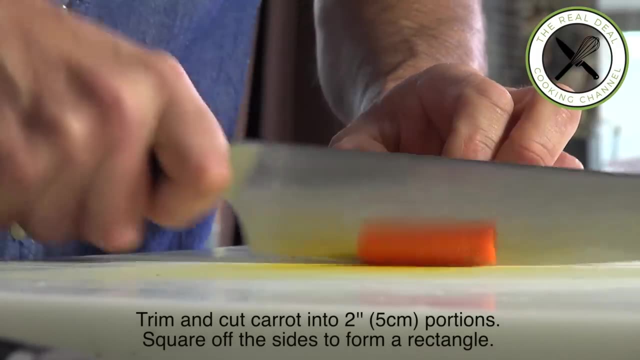 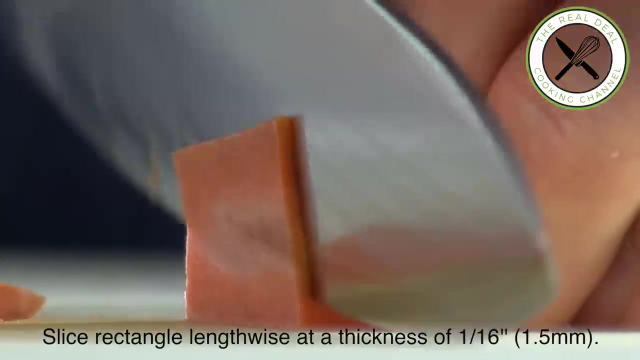 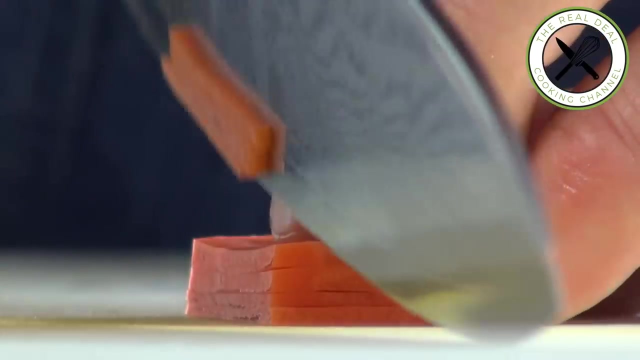 one, then cutting a vegetable into fine brunoise or very fine dice. One and a half millimeter cuts, so great for garnishing and stuffing. The first step here is to square off the item. then slice that rectangle lengthwise at a thickness of 1 16th inch, 1.2 millimeter. 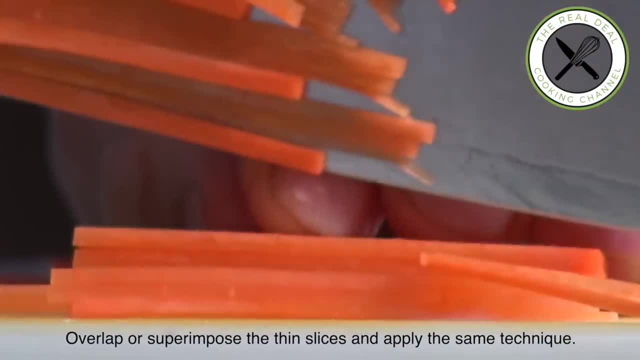 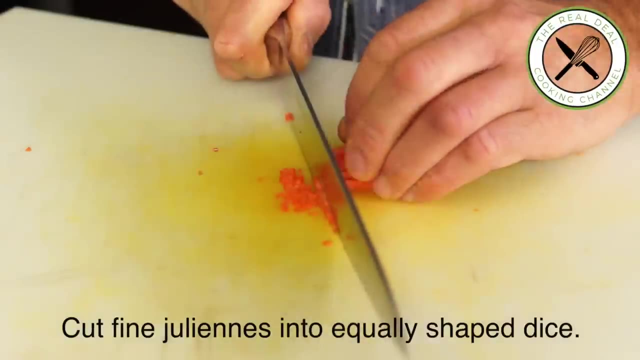 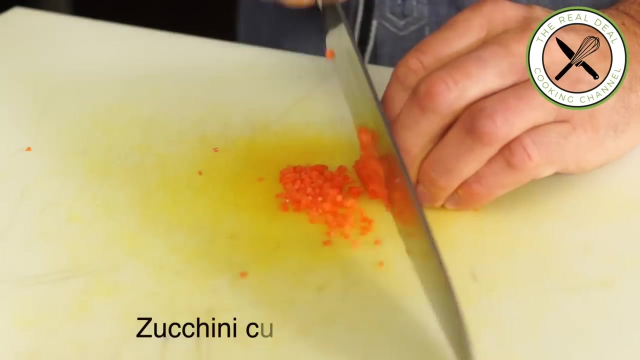 leaving you with rectangular cuts. Then overlap or superimpose the thin slices and apply the same technique. You will end up with fine julienne. then cut this julienne into equally shaped dice. Next, brunoise, a twice bigger cut than the fine. 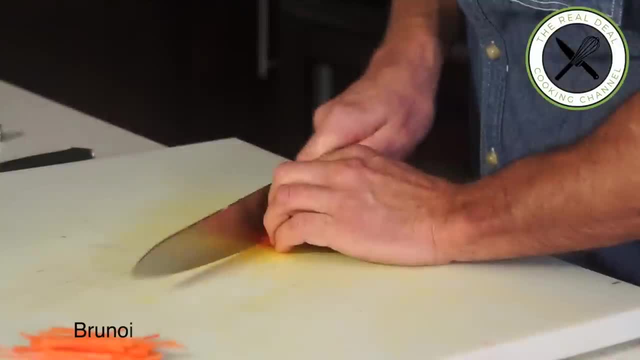 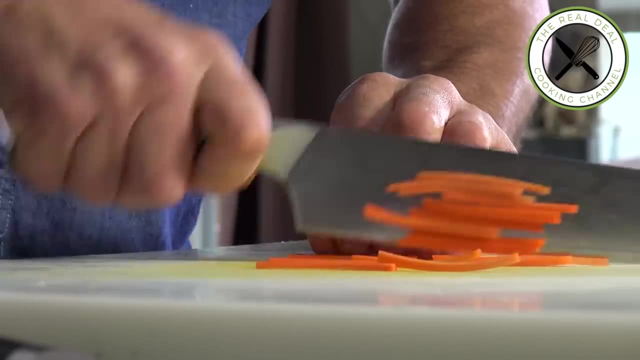 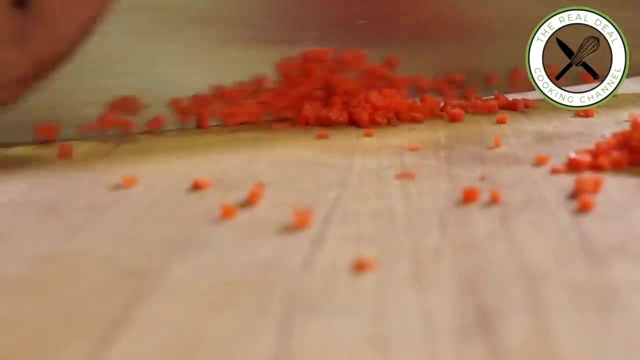 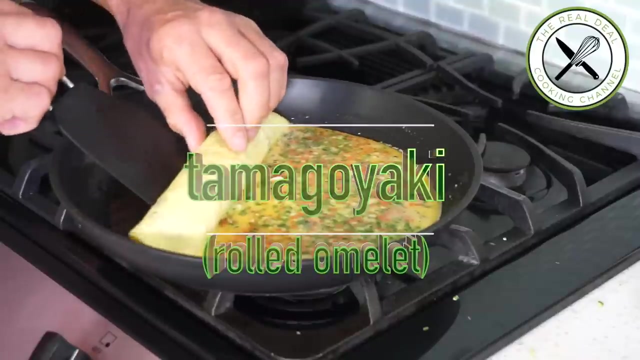 brunoise size, measuring approximately 1, 8 inch, 3 millimeter. Julienne or allumette or matchsticks, such as spring and summer rolls, or diced for stunning salad stuffing, And this superb tamagoyaki, a Japanese style rolled omelet. Look at that. 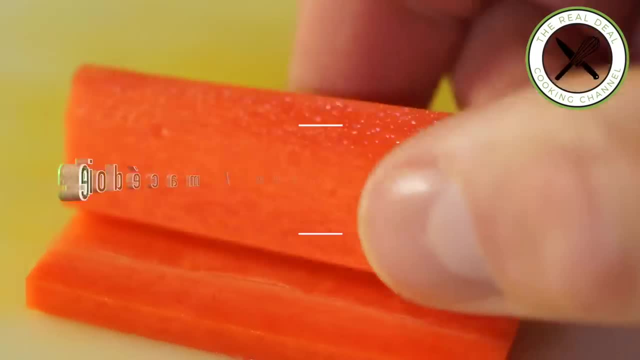 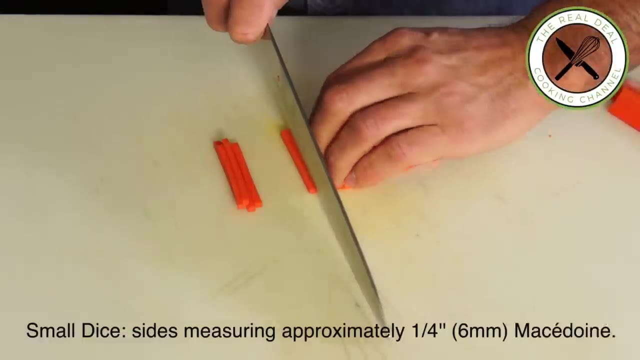 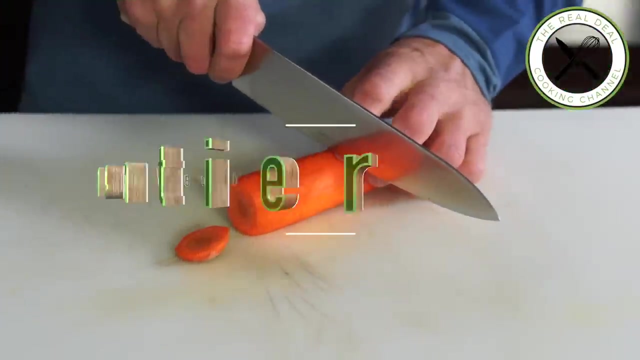 Next and third, cut twice bigger in size than the brunoise. 1 quarter-inch. 6 millimeter slices cut into batonaise produce small dice or massive ones. For the 4th, cut twice bigger in size than the massive one called medium dice or parmentier- Same principle trim. 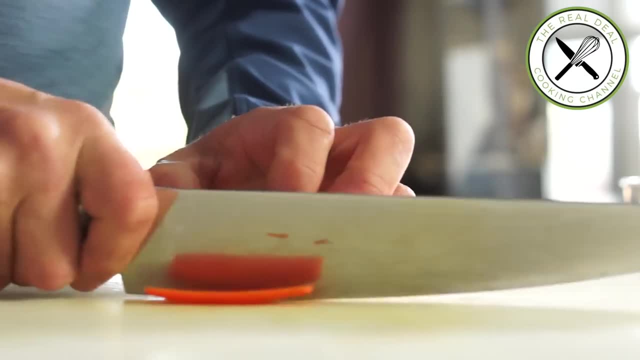 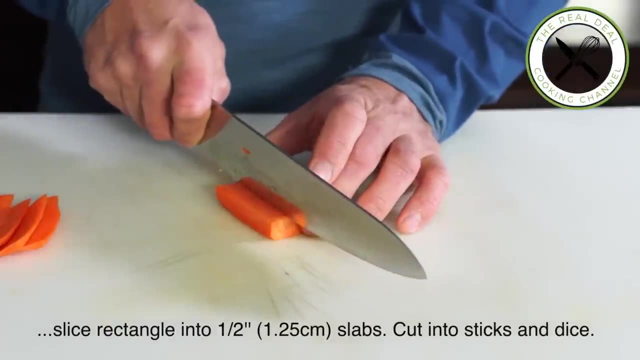 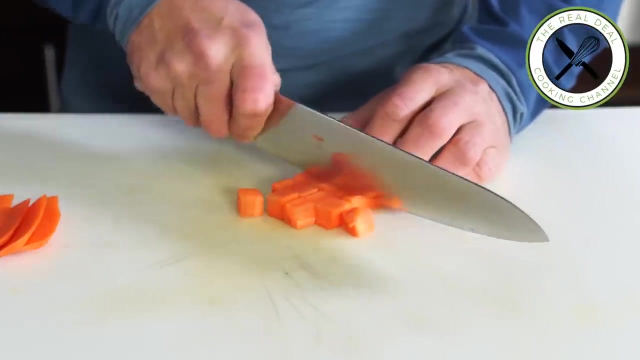 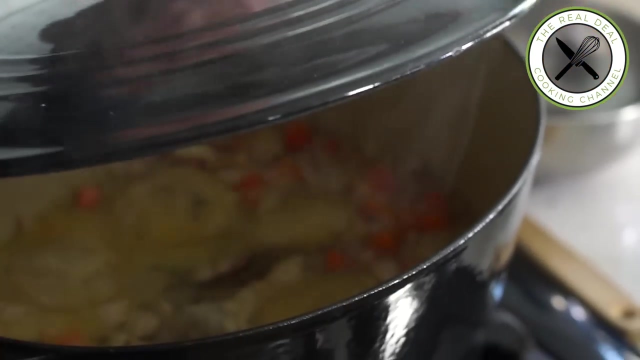 and cut carrots into 2 inch, 5 centimeter portions, Square off the sides to form a rectangle, just like we did before. Slice rectangle lengthwise at a thickness of half inch- 1.2 centimeter and cut slabs into half inch batonnes and dice out And take a look at what you can do with. 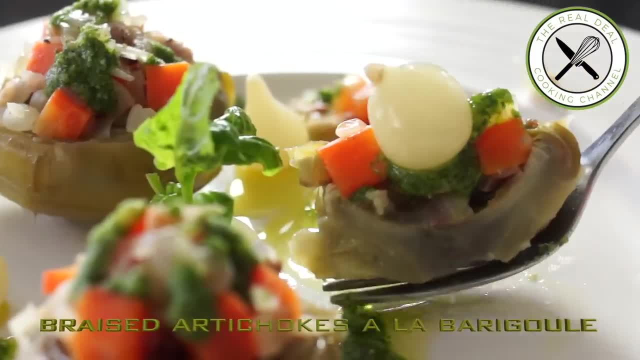 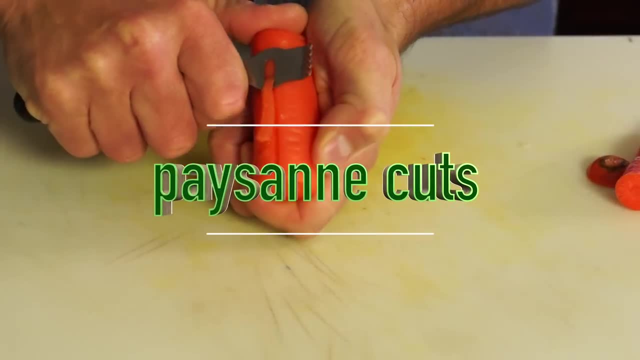 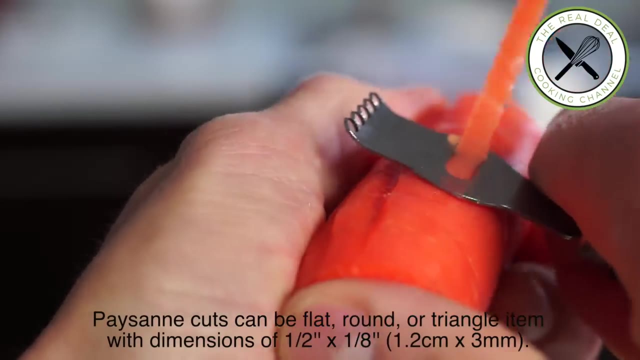 these little cubes, braised artichokes à la barrigoule, So delicious. Next, peasant cuts. These can be flat, round or triangle. Let's be fancy for that one, and I'm gonna use a lemon zester grater. And then I'm going to build my own old clock.